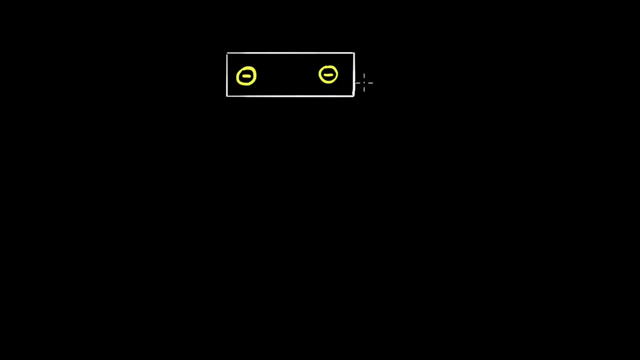 them. And let me call that picture, let me call this arrangement as arrangement one. So we start at rest. That's important. We start at rest. And now what's going to happen? Well, I know that if I wait for some time, these two electrons would have gone slightly farther apart. okay, And they'll keep. 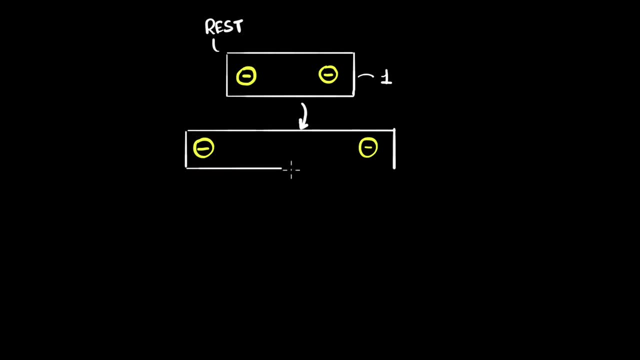 moving. But again, I'll take some action. So let me take a picture at this point And let me call that picture as arrangement two. Okay, Let me define what a stability and instability is. okay, Are you ready? Okay, We say this: arrangement two is more stable than. 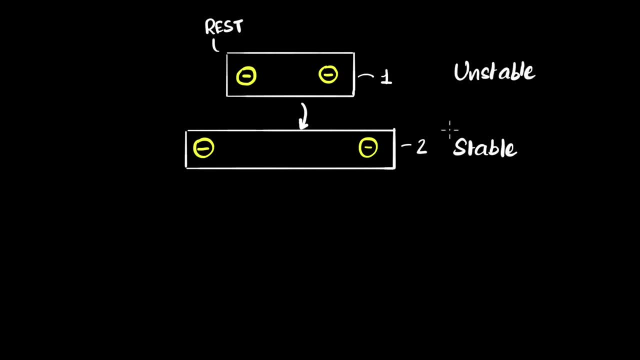 arrangement one. We say arrangement one is unstable. arrangement two is more stable. Why? Because, by definition, the meaning of stability is: you take a set of particles at rest, let them go, and then you take a set of particles at rest. Whatever new arrangement comes, by definition that is stable. That's, that's all there is to it. Are you thinking? is that simple? Yes, Whatever fancy definitions your textbook must be giving you at the heart of it, this is what we mean by stable and unstable. Let me give you one quick another example. Two examples are better than one. Let's say I have two charges this time, one positive, one negative. Again, I start them at rest. 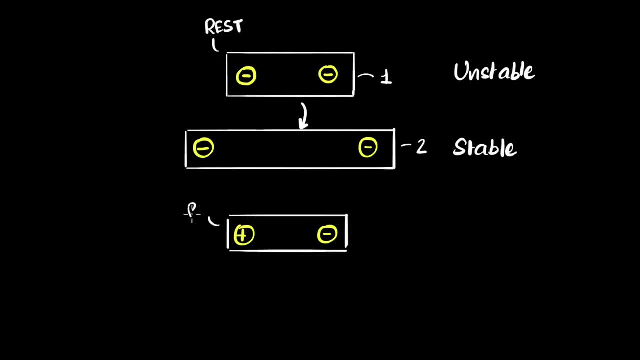 Let them be at rest to begin with. rest arrangement one: Okay, this is second example. So I'm going to put a line over here. All right, Now let them go. What's going to happen? Well, they are going to attract each other. After some time. they would have come closer to each other, Okay, But I come closer to each other Now. again, by definition, I let them go. Now I have a new arrangement. They were at rest. Now I have a new arrangement. So what I'm going to do is I'm going to 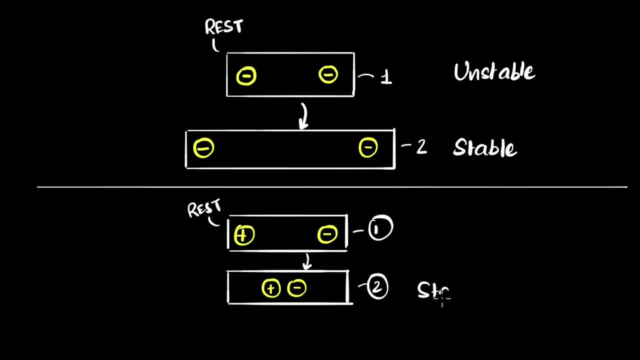 So, whatever happens, whatever new arrangement you get, by definition is more stable compared to this. So this is unstable and this is stable. Why do we say that? Well, we say that because we like to personify nature. we like to think with our emotions. 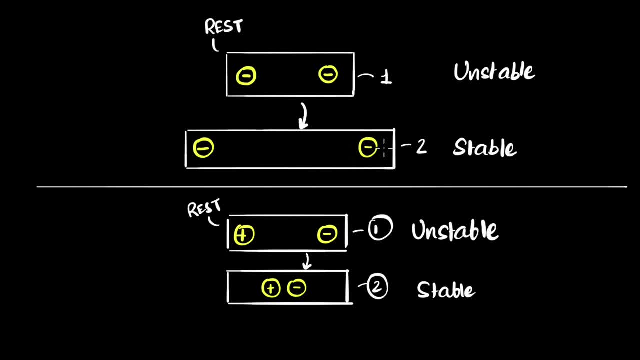 and we like to say: nature has a preference. and we say that two, arrangement two, is more preferred to arrangement one. And the way to test this in your head is we can say: if you start this at rest, we get this. 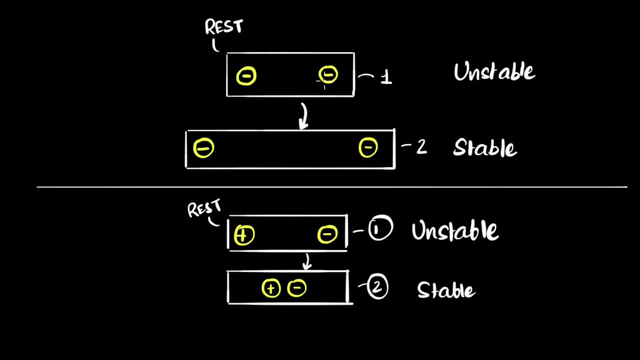 But if you had started this at rest, would you get this? No, you wouldn't get this right. Therefore, nature prefers two over one and therefore we say: this is two is more stable compared to one. Same thing over here. 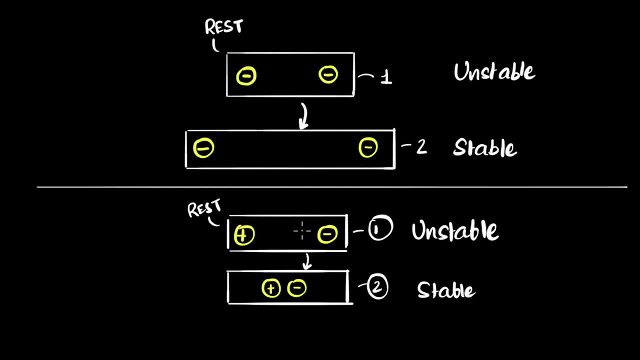 If you had started with this at rest, you wouldn't have gotten this, But when you start this at rest, you did get this, So nature prefers two over one. therefore, this is more stable compared to this, and that's all there is to it. 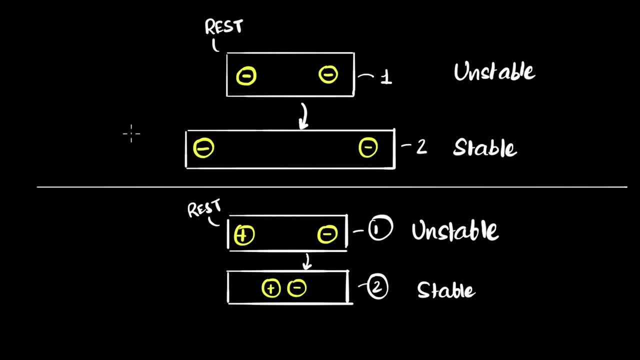 So if you take your emotions out, if you think about preferences, you take them out. then what is stability? How do you know if something is stable or not? Take a system of particles at rest. let them go. whatever new arrangement you get is stable. 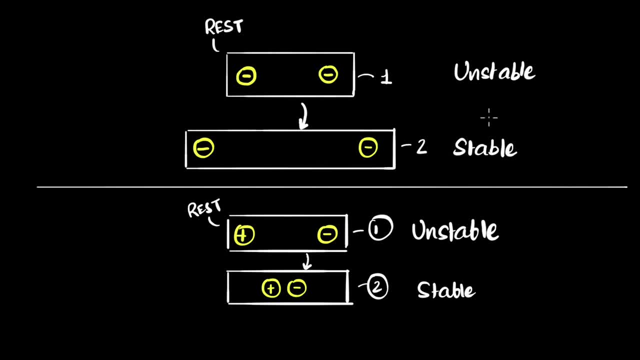 That's it. that's all there is to it. Now. just from this, one thing you can immediately see is that the terms stable and unstable are relative terms. I can only say that one is unstable compared to two. I can only say two is stable compared to one. 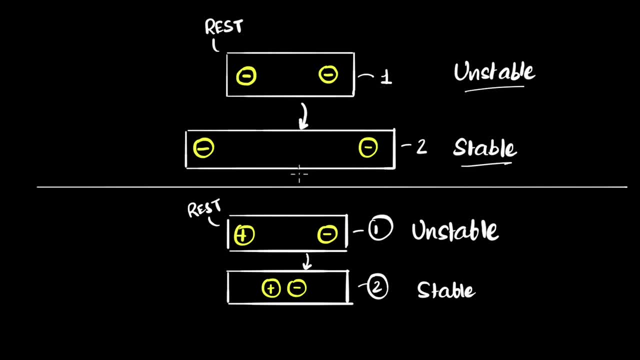 If I just look at two and I ask you: is this stable or not? that question makes no sense. Stability and instability are only talked in terms of relative. like you have to compare it Same thing over here And that's why I absolutely hate it when in chemistry 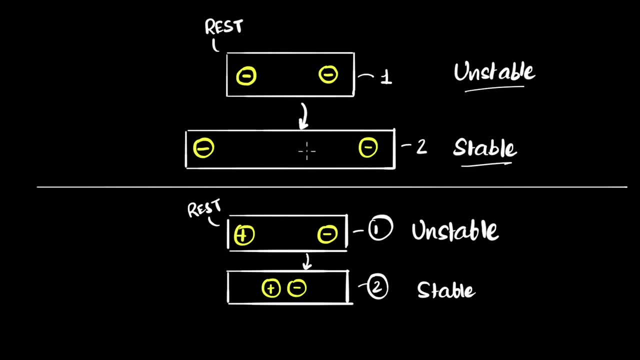 I get annoyed in chemistry when people say that hey, you know what these molecules are stable, You know what these molecules are unstable. I get annoyed because I say: unstable compared to what, Stable compared to what to what? now, sometimes it's like understood. for example, if you're talking about the stability of 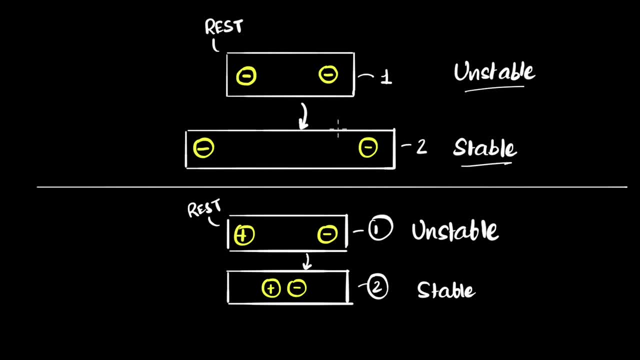 the products. we are comparing it with the stability of the reactants, for example. that's what it is, but you need to be always sure what you're talking about. otherwise, what can happen is is that stable and unstable are terms we use in our daily lives and they have very loose meanings. we don't think. 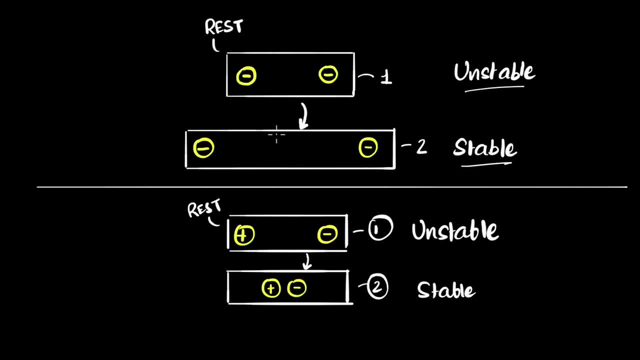 about what really they mean, and so when we use them in science, it gives us a feeling as if we have understood it. it we feel like, ah, that makes sense, whereas in reality you wouldn't. and that's why it's super, super important to be very clear, crystal clear, with what it means to be stable and 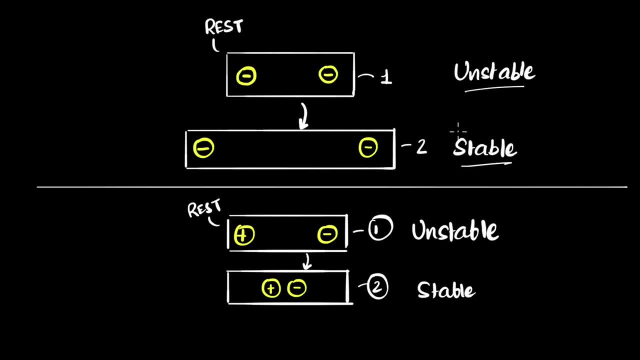 unstable. and now that you understand it, always remember, whenever someone talks about stable and unstable, always ask them: compared to what always ask yourself. i'm comparing this system with respect to what? okay, there's a second thing i want to clarify. there is idea of stable and unstable. 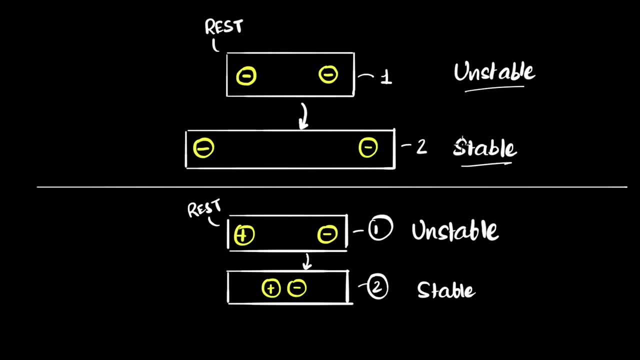 equilibrium. that's a completely different. that's a slightly oh, it's a different thing. it's a different thing. i can look at a system and i can say, aha, that's at stable equilibrium. i don't have to compare it to anything and i can look at a system. 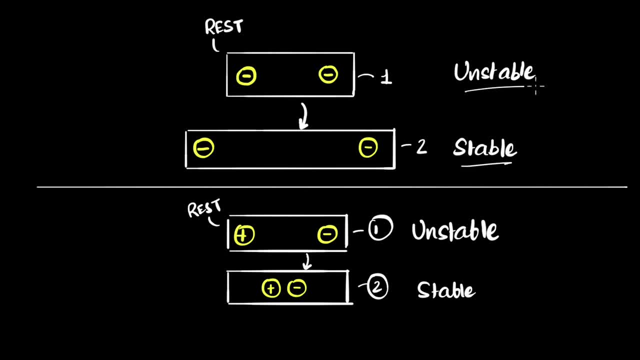 and i can say: aha, that's unstable equilibrium. that's a completely different thing altogether. i'm not talking about that, but let me know if you want to talk, want me to talk about that. i can cover that separately in a separate video, but that's a completely separate thing. these are not things. 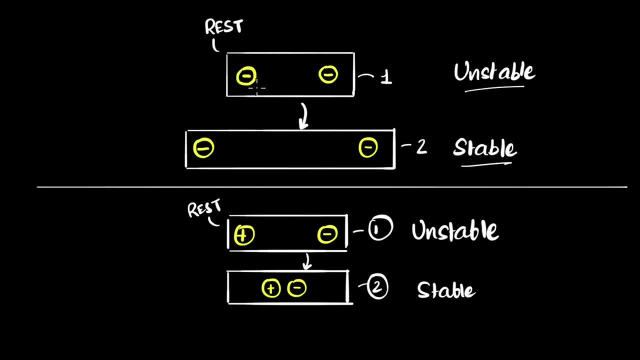 at equilibrium. equilibrium equilibrium means balanced forces or no net force. here there are net force forces, so we're not talking about equilibrium. okay, now let's connect it to energies. my first question to you is: as i go from system one, arrangement one, to arrangement two, what do you? 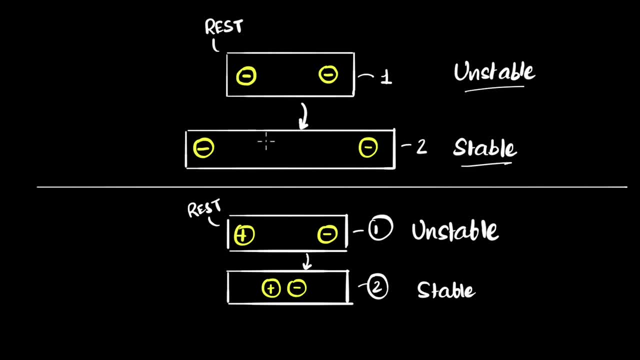 think happens to the total energy of the particles. don't worry about whatever you've learned so far. just use some. just use first principles and see whether you can answer this question. okay, the thing that i'm going to use is law of energy conservation. it says that energy can. 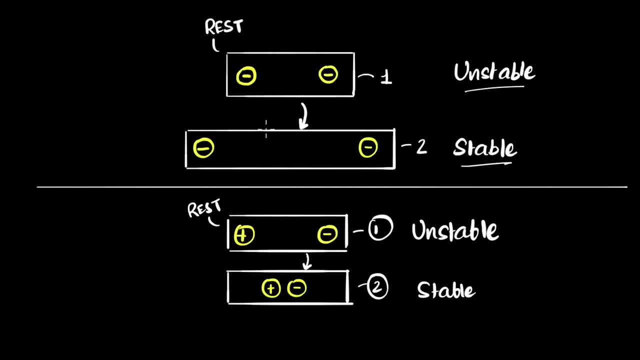 either be created nor destroyed. when i went from here to here, okay, the total energy over here, i'm going to ask myself: did energy get added or removed? and the answer is no, it's a vacuum. let's imagine that there was no energy added, no energy removed. the total energy must stay the same. so the 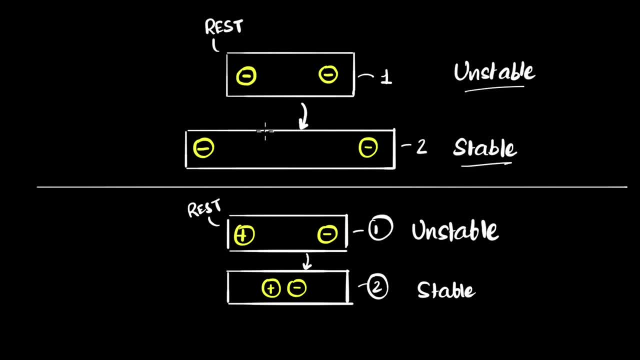 total energy did not change. however, if you look at the kinetic energy, that has definitely changed. see, initially the kinetic energy was zero, but when i went from here to here, the particles are now moving. they're moving away from each other. they have some speed. therefore, the kinetic energy is. 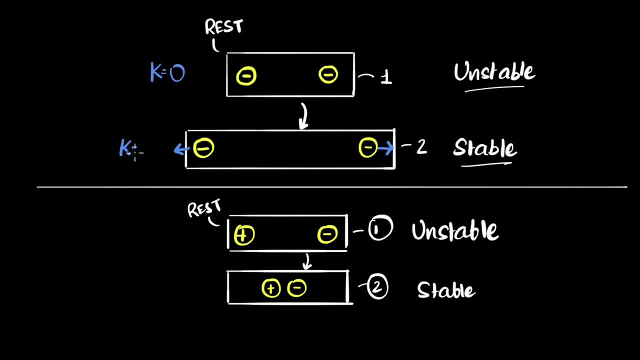 not zero. so let's say that kinetic energy is some number. let's call that 20. the question we could ask is: hey, where did this 20 energy come from? because energy can neither be created nor destroyed. oh, that's where we cook up this new idea called as potential energy. we say that, hey, you know what? 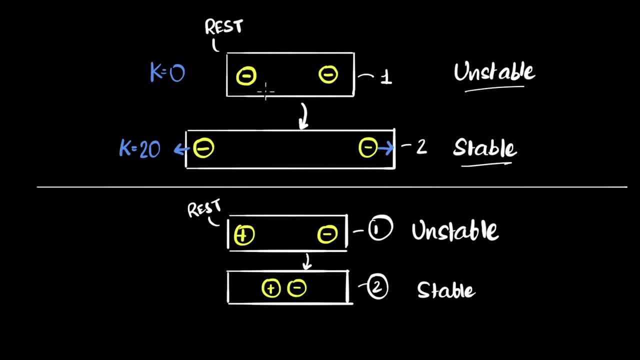 there was some energy stored over here, not in terms of kinetic energy, it was stored. the arrangement itself has this energy. it's the energy of the. the very configuration has an energy. we call that as potential energy. but we said when we went from here to here, we said that there was some energy. 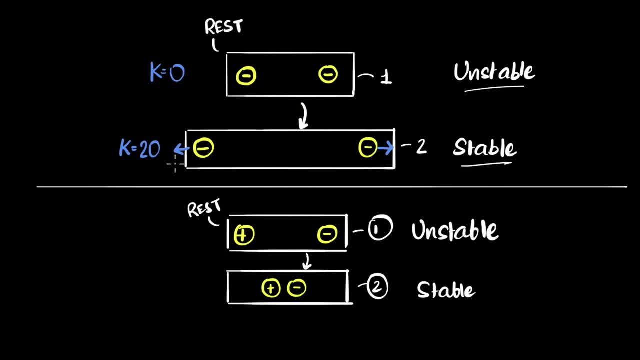 that was converted into kinetic energy and that's where that kinetic energy came from. and therefore over here we had some potential energy and let's just again give some number to it. let's say the potential energy was 100 to begin with. then we say that out of that, 20 got converted into kinetic. 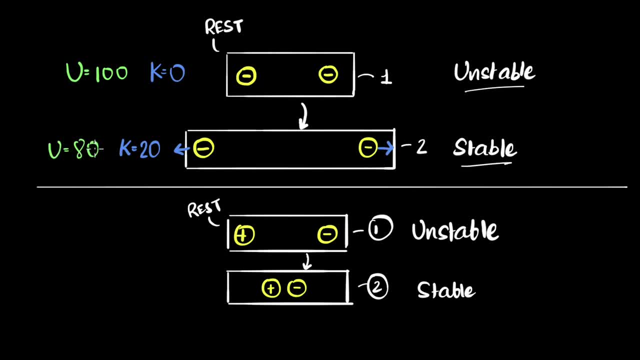 energy, and so the new potential energy now has to be 80, because total energy has to be conserved. and so notice what happened when i went from here to here. notice what happened to the potential energy. what happened? hey, it reduced, potential energy reduced. and notice when i went from us, when 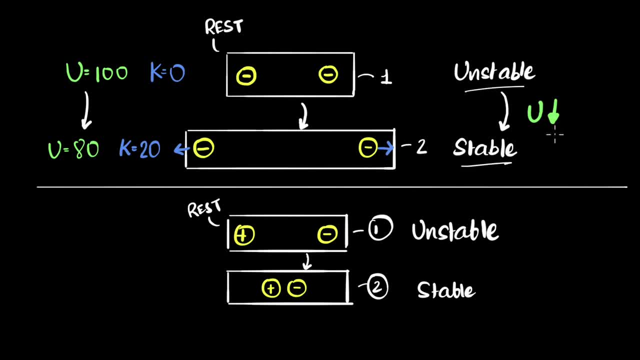 i. when i went towards a more stable arrangement, the potential energy lowered. let's see if the same thing happens over here. i start from rest when i go from here to here. clearly they're going to have, they'll be moving towards each other and therefore they will have some kinetic energy. so 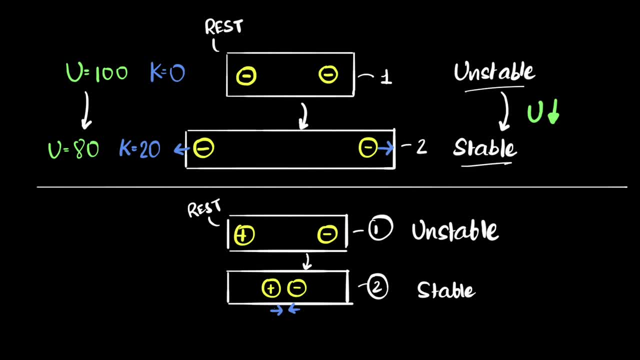 is this: my potential energy reduced or decreased? why do i have that reduced? potential energy is so increased. oh wow, potential energy must have reduced. can you see how this makes sense? now, when i go towards stability, when i go towards stability, potential energy must reduce. why? because i start from rest and when, when i go towards stability, when, when, when time progresses, whatever, 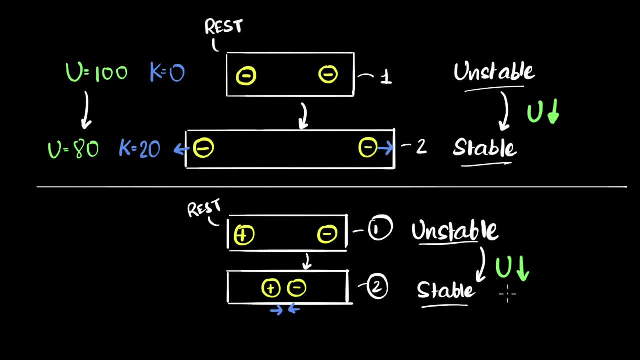 they started moving and because they started moving, kinetic energy increased. therefore potential energy has reduced. and that's why, when you have a more stable, when you're going towards more stability, the potential energy gets lowered. and that's why stable systems have lower potential energy compared- always compared compared to unstable systems. does that make sense now? 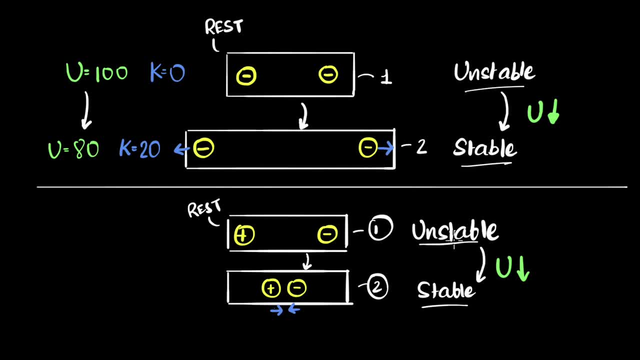 that's all there is to it. that's all there is to it. but you may ask mahesh then: but why do we talk about potential energy? why not talk about? okay, there might be several questions for you. one question could be: why are you talking in terms of potential energy? why not talk in terms of? 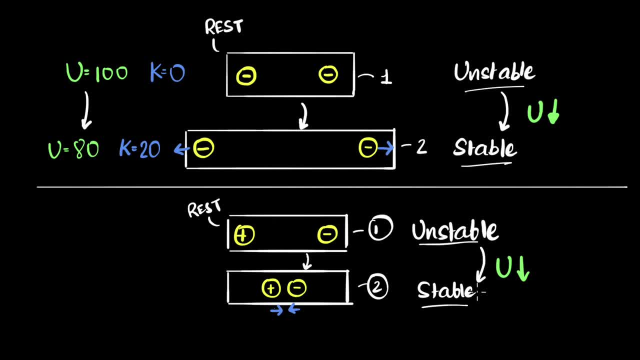 kinetic energy. why do we say that, hey, when you go towards stability, the kinetic energy increase. why can i say that? the reason you can't say that is because kinetic energy can be converted to something else, for example, in this case, if you were in vacuum. this is the 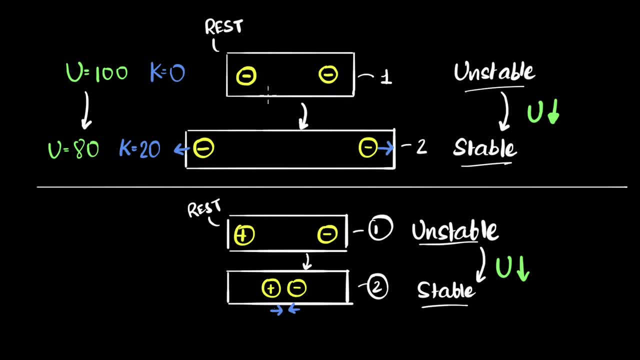 problem. this is the situation. but imagine these were two tennis balls- negatively charged tennis balls, kept in water. i don't know who would do that and why you would. anybody would do that, except for when you're conducting some science, hypothetical science, experiments. but if this was in water? 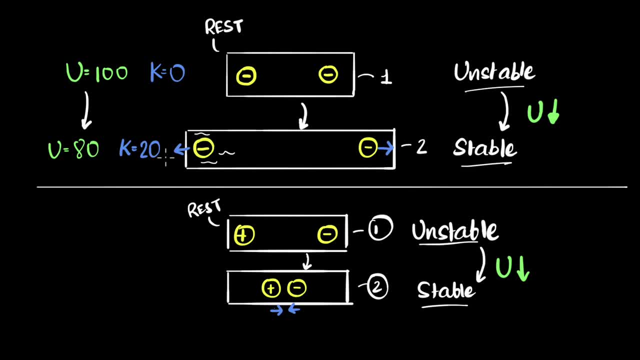 then what would have happened is that the it would, it would collide with the water particles and it would dissipate energy, so that kinetic energy would get converted into heat energy. okay, and so now what would happen in arrangement two is that the kinetic energy would have actually gone to zero. 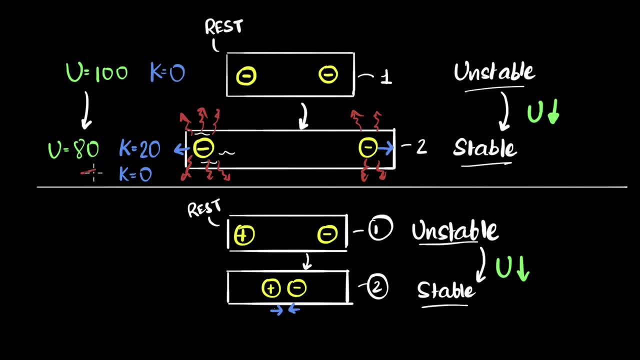 and all that energy would have been converted to thermal energy. so you would have now thermal energy, that that all that kinetic energy would have gone to thermal energy. so would it be accurate to say that when i go from an unstable system to stable system in general, that kinetic 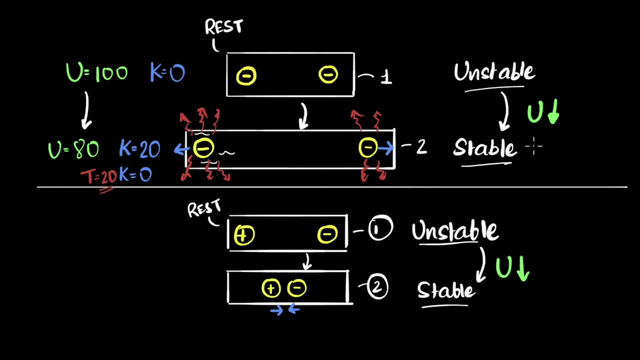 energy increases? no, but would it be accurate to say that the potential energy decreases? yes, because whether the kinetic energy increases or not, or whether the kinetic energy has got transfer to thermal energy, light energy, sound energy, whatever energy it is, it comes at the expense of potential energy. 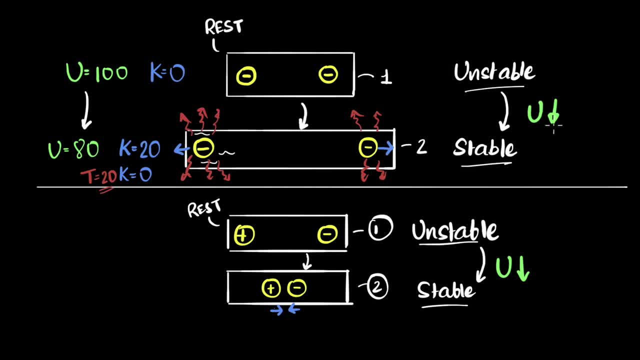 And therefore I know for sure, with 100% certainty, in general, the potential energy must have reduced. That's why we talk in terms of potential energy. We just forget to say it sometimes and therefore we just use the word energy and we say hey. 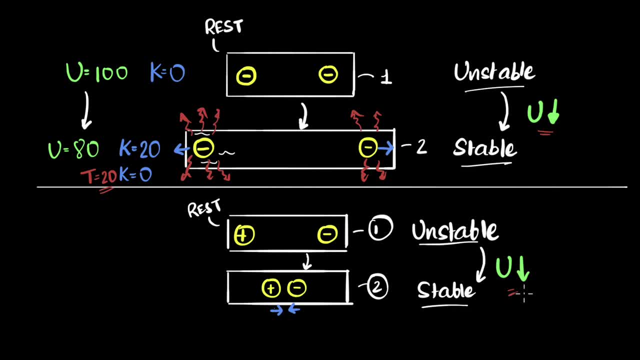 stable systems have less energy. But remember we're always talking about potential energy. when we say that, The last question you might have is: but Mahesh, why do I need this in the first place? Why do I need to talk about energies in the first place? 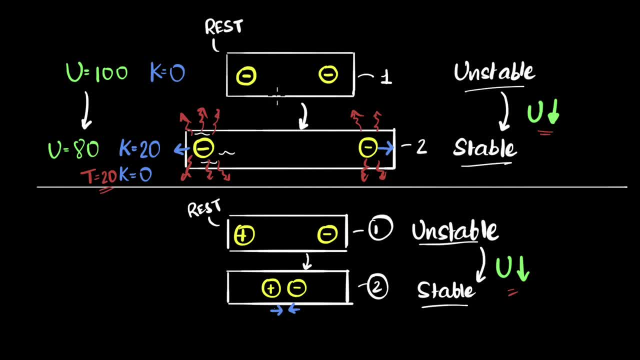 I know just by looking at the situation whether something is stable or unstable. I can compare and I can do that right? True, you can only do that if you started with things at rest. Remember that's how we thought about stable and unstable. 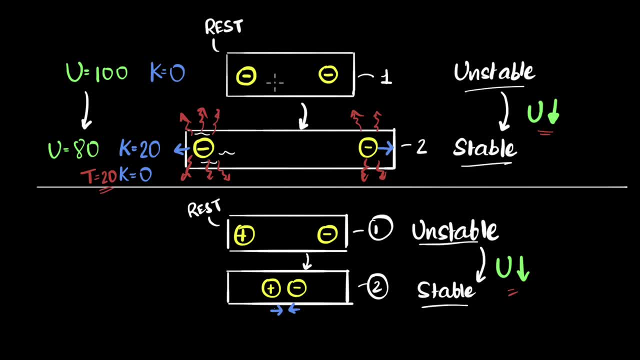 When things are starting at rest, then I know for sure whatever happens goes towards stability. But what if things are not starting with the rest? Then how do you do it? And things can be complicated. Then the best way is to look at what happens to your potential energy. 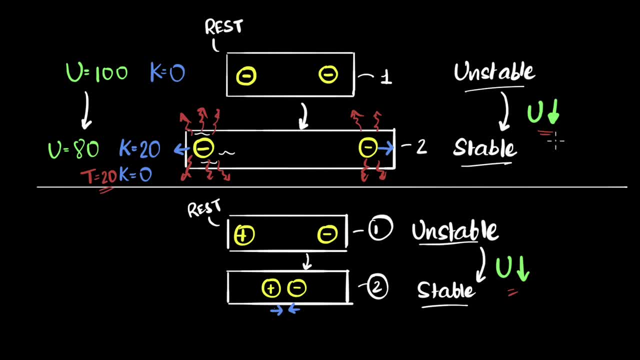 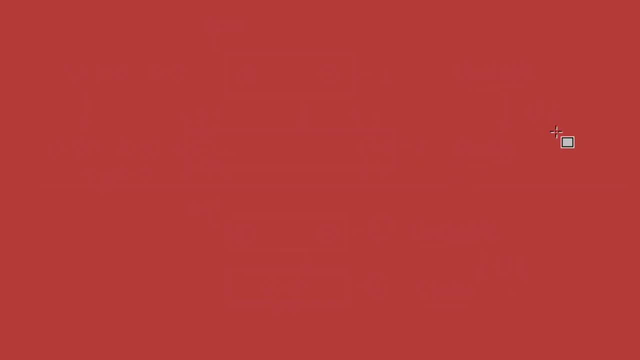 If it is lowered, you know that system has become stable. If it increases, you know the system has become more unstable. So let me give you the one last example, and then let's wind this up. Oops, I went black, Okay. 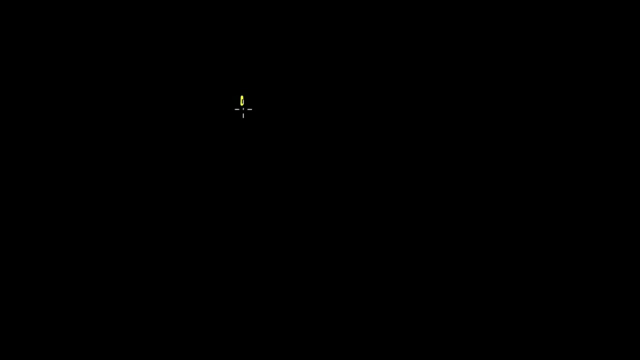 All right. So let's imagine that I have a positive charge, a negative charge To begin with, And they are moving away from each other. They have some speed and they are moving away from each other And let's say: this is our arrangement 1.. 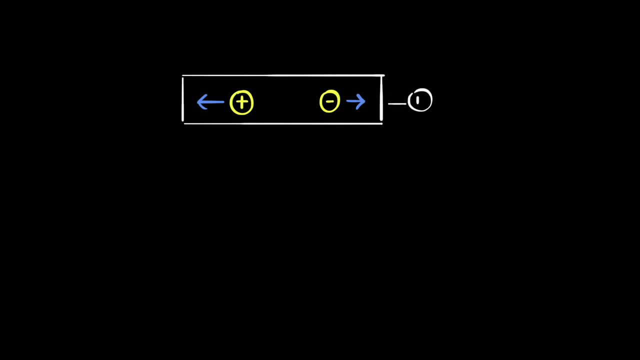 Oops, Okay, This is our arrangement. 1. After some time they would have moved away, And let's call this as our arrangement. 2. Now I ask you, what happened to the stability? Is this more stable? Less stable? 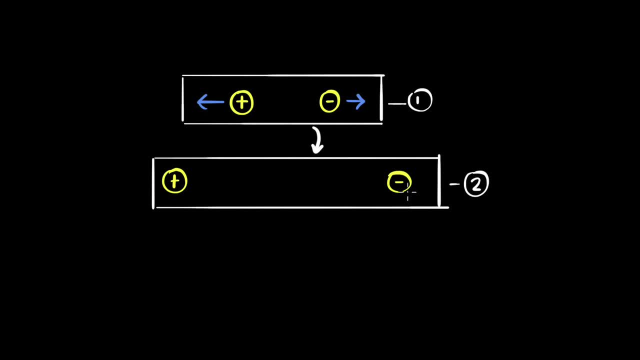 What has happened Now? can I say that As time progresses, things become more stable? I can't say that because I didn't start with rest. That can only apply when you start with rest. Okay, That simple definition of stability and instability. 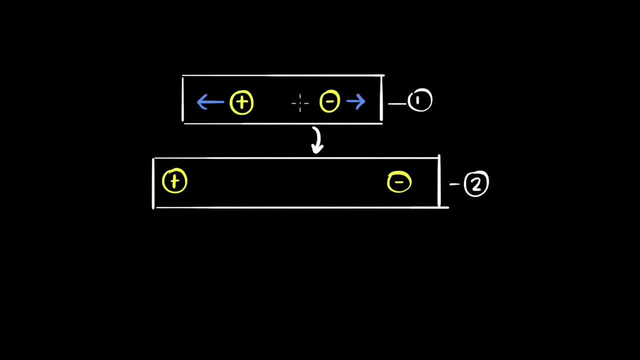 Now that I haven't started with rest, I can no longer say that. So what do I do? Look at potential energy. Okay, So I start with. this has some total energy, and I know that this total energy stays the same, I'm going to assume everything is in vacuum. 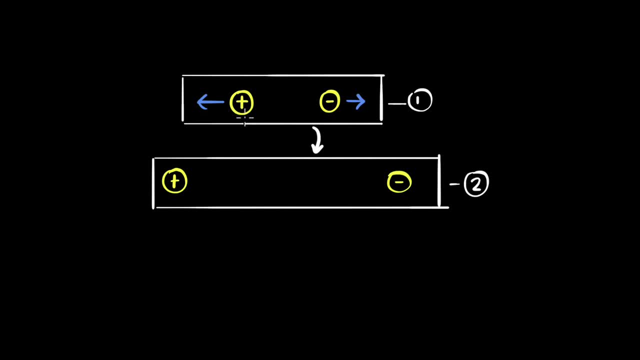 But I know I'm going to look at kinetic energy and that's how I actually get a clue of what happens to potential energy When I go from here to here, what happens to kinetic energy. This has some kinetic energy, But as I go from here to here, notice that they are attracting each other. 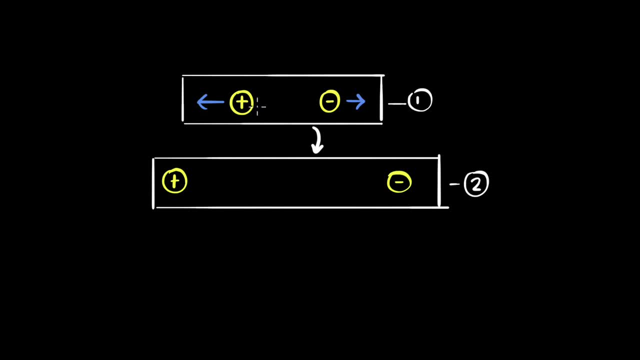 They want to come closer to each other And because of the attraction, you know the experience of force- I'm going to use pink color to draw the force. Notice: the force is this way, The velocity is this way. Clearly they're going to slow down. 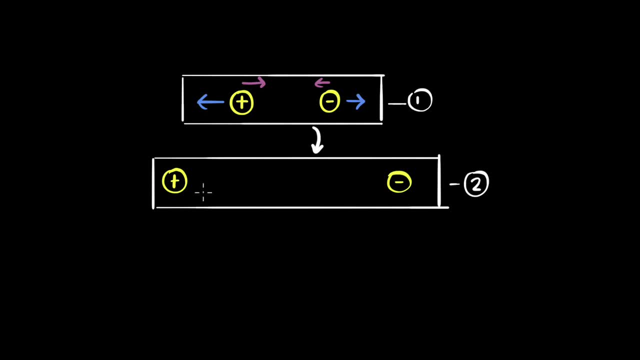 It's kind of like throwing a ball up right Against gravity. it slows down Against the electrostatic force. these slow down. So what has happened to their speed Decreased? What has happened to their kinetic energy Decreased.